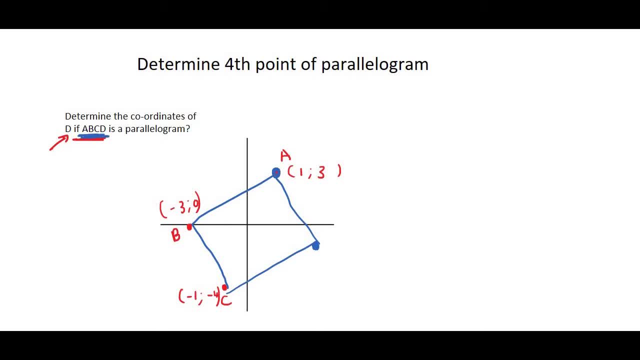 like a rectangle. that's okay. Rectangles are also parallelograms, So D would be somewhere over here. Now, all that you do, it's very easy. you just look at B going to A, for example. How did the X values change? 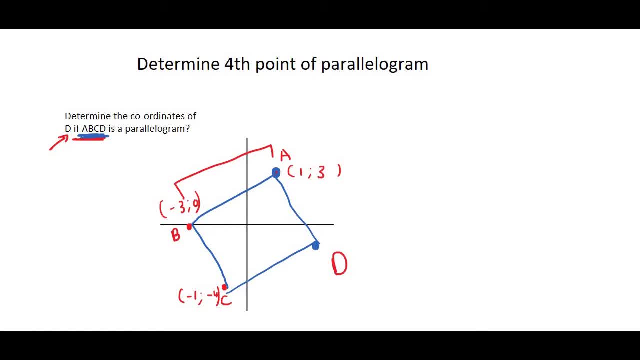 Well, from B to A, the X values increased by 4 because they went from minus 3 to 1.. So we do the same with this coordinate: If you add 4, then this X value will become 3 and then the Y value went. 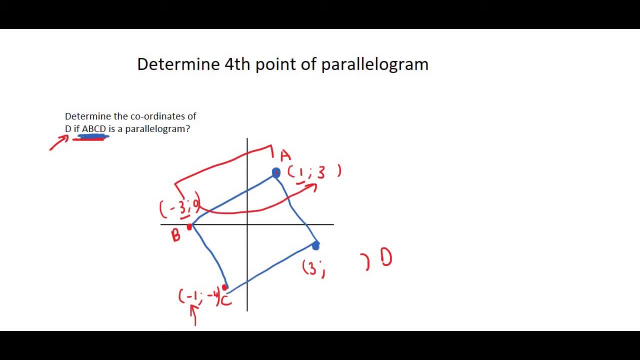 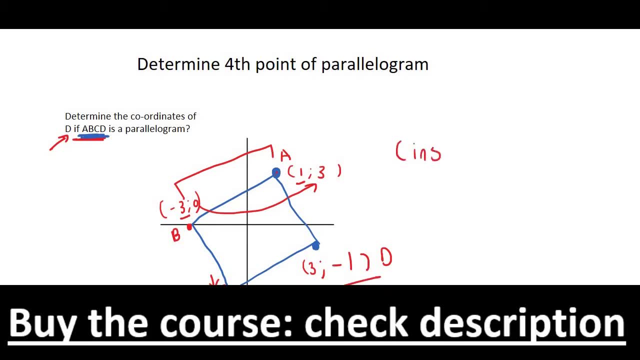 from 0 to 3, so that means it went up by 3.. So you do the same to this: minus 4 and that'll be minus 1.. And there we go In a test. your reason would either say: inspection- some teachers do that. 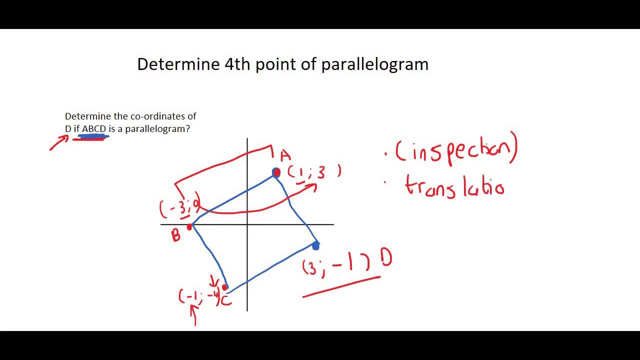 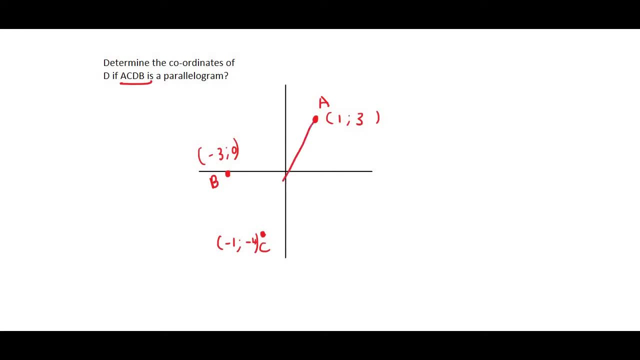 or say translation. So just see what your teacher says and stick with that. Here's another example, but now the order is different. It's A, C, D, B, So it goes from A to C, then to D- which we don't know where it is, which is going to make things a bit confusing- and then to B. So what I would do is I: 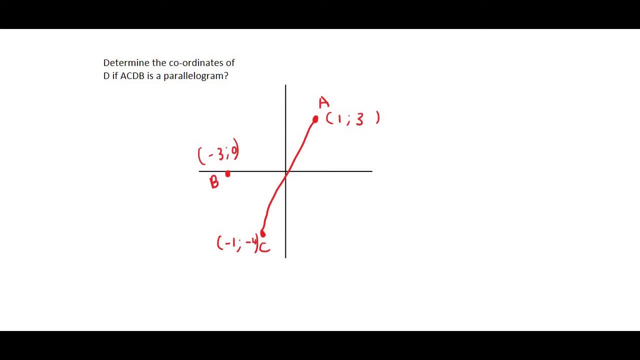 would connect these two so long, because we know that B is going to eventually connect to A, because B is the last letter, and then it would have to go back to A. I would then make a line parallel to this one, so it would go somewhere like that, and then I would. 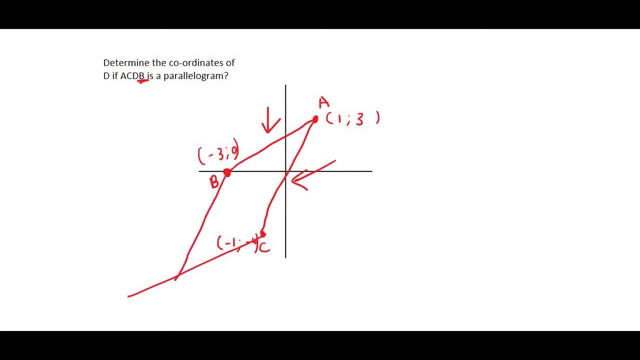 make a line parallel to this one, which would go something like that: So D would have to be over here. Now it's very easy. What I do is, for example, I look at this coordinate and I see how does it change to go to there. You could, even, if you wanted to, you could look at this coordinate. 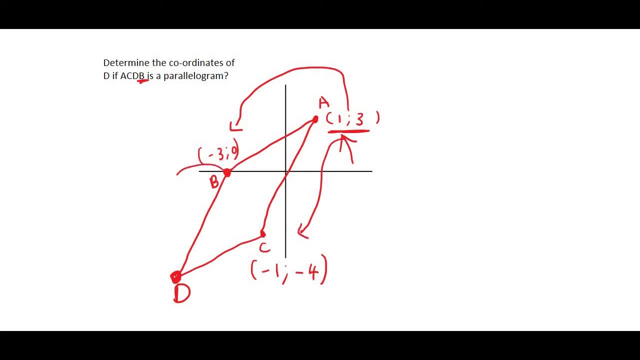 and see how it changes when going downwards. Then you could do the same from B to D. It doesn't really matter. But what I'm going to do is look at going from A to B. So it looks like the X value went from 1 to. 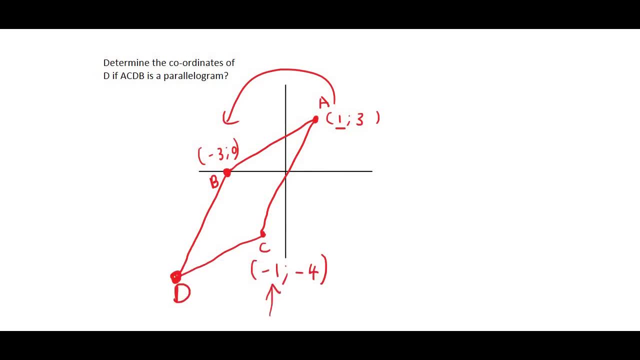 minus 3.. So it goes down by 4.. So if we let this go down by 4, it will go to minus 5. and then the Y value went from 3 to 0. So it goes down by 3.. So this one must go down by 3.. So it'll become minus. 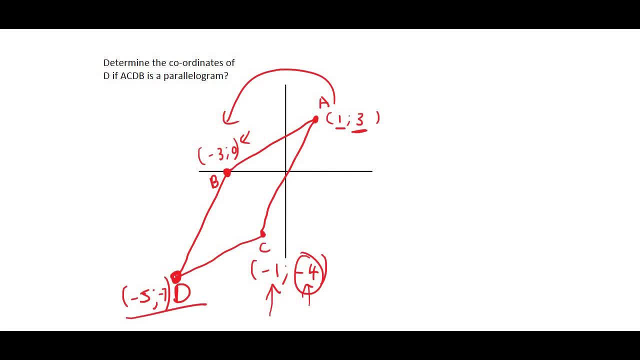 7, and there's the answer Once again. your reason would be inspection or translation.